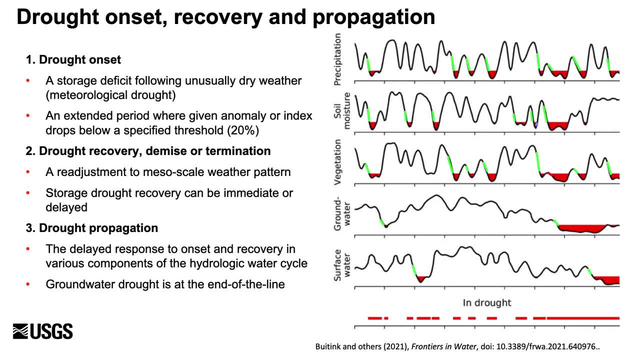 below a specified threshold indicating the start of drought Recovery is the period of positive anomaly increase terminating the drought. Each hydrological system may have a different onset and recovery period, as well as different rates of change as drought onset and recovery propagate to the whole system. The rate and lag of onset and recovery and the propagation from precipitation. 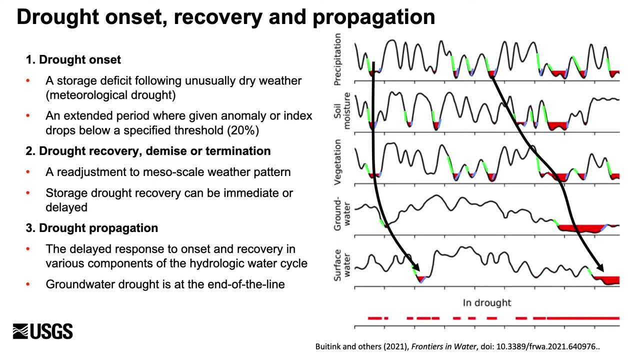 to groundwater within a given basin can provide information on watershed resiliency and vulnerability. A last note on this figure: while drought events are, by definition, extreme events, drought occurrence across the entire hydrological system is a relatively common feature. Some components are almost always in drought, regardless of the others. Monitoring wells. 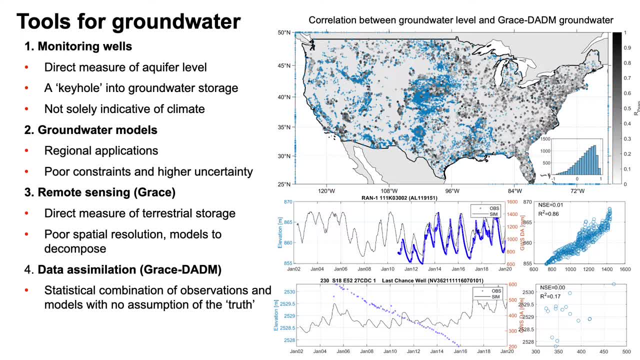 perhaps the most direct evidence of groundwater drought. However, the time series of levels can be short, sporadic and incomplete in national groundwater databases such as the National Water Information System and the National Groundwater Monitoring Network. Wells provide a keyhole into the aquifer. 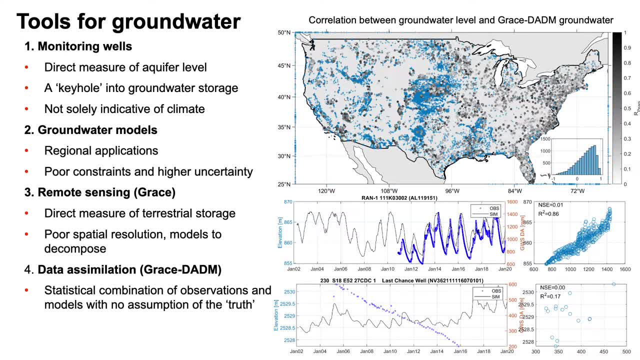 but not necessarily a direct observation of aquifer storage or response to drought. Observation wells are not always in shallow and confined aquifers directly recharged by precipitation. Wells are more often in areas of significant groundwater withdrawal for irrigation, and drought may likely increase such withdrawals. 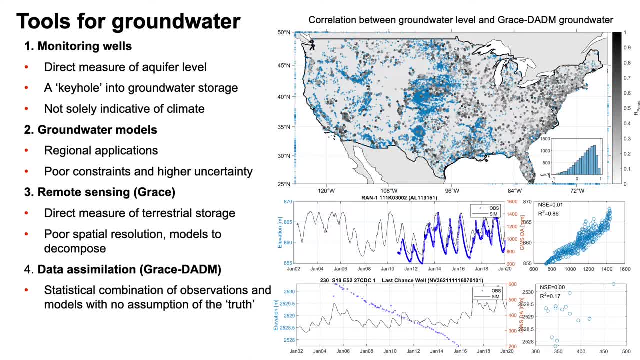 Models, on the other hand, estimate aquifer storage and are generally constrained by precipitation and stream flow, but many other uncertainties in these models are often lumped into groundwater storage. Remote sensing, primarily through NASA's GRACE satellite, provides a direct measure of total water storage. 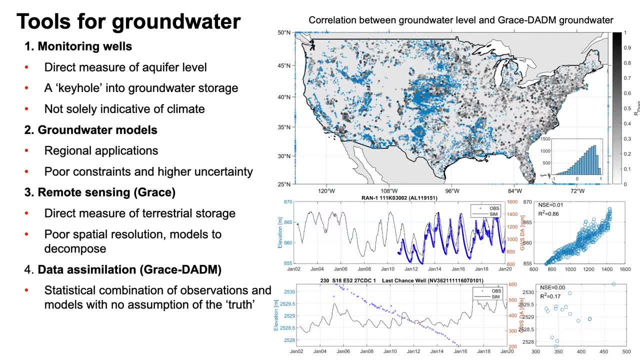 but requires models to disaggregate these gravity anomalies into changes in groundwater storage, and the spatial resolution is very coarse. Finally, data assimilation blends models and observations from satellite and in situ data to statistically push the models towards observations and reduce model uncertainty and bias. 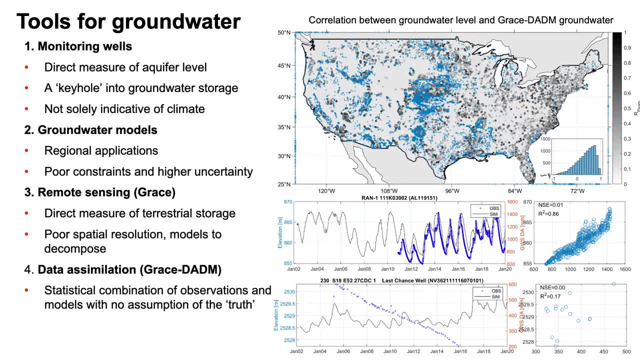 The top right figure shows the correlation between shallow groundwater storage from the GRACE data assimilation product and over 4,000 observation wells with more than 10 years of data. Darker symbols show wells with higher correlation to GRACE, indicating a greater coupling to atmospheric conditions. 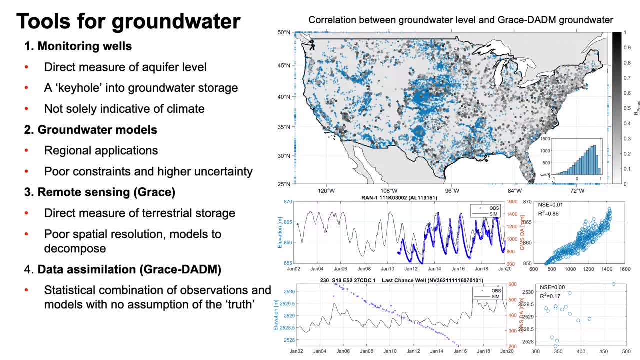 Note the scatter with the high correlation for a well in Alabama. The blue crosses on the map indicate no significant correlation such as shown in the lower scatter plot of the last chance well in Nevada. Here groundwater mining is lowering levels independent of drought, While GRACE does measure groundwater withdrawal. 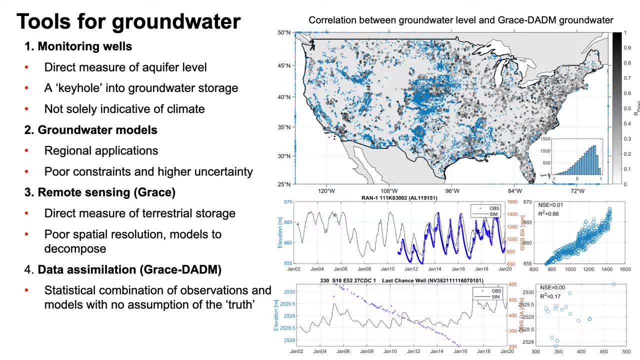 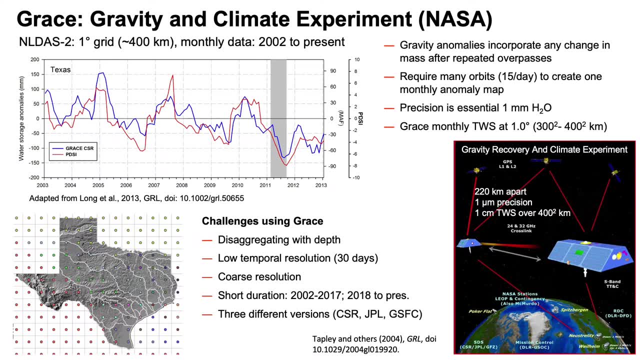 data assimilation cannot fully adjust these models for such human-induced changes to the water balance. Monthly maps of terrestrial water storage change are constructed from NASA's Gravity Recovery and Climate Experiment and the GRACE follow-on satellites, which detect small changes in the Earth's water storage. 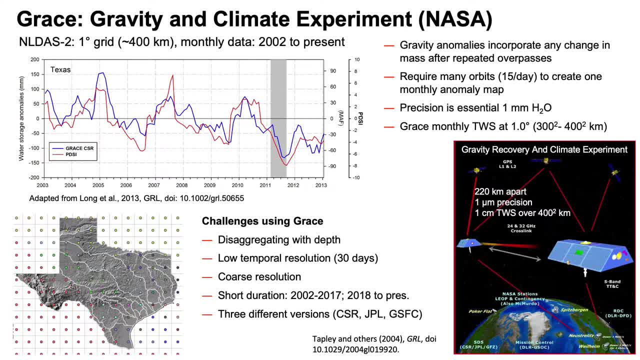 Water storage is getting more expensive with the use of ground and groundwater storage systems, including those in areas where there are relatively small differences in the Earth's gravity field caused by the redistribution of water on and beneath the land surface. Paired satellites travel about 140 miles apart. 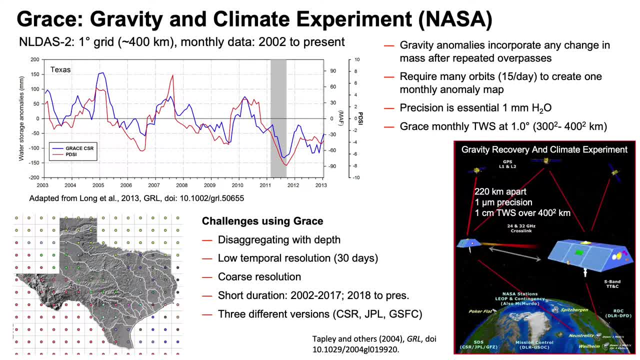 at an altitude of 300 miles and record small changes in the distance separating them as they encounter variations in the Earth's gravity field. The vertical extent is measured in centimeters of equivalent water thickness, which is mostly related to near-surface water storage. 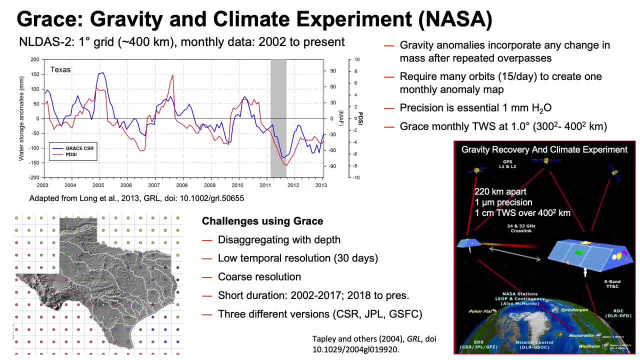 in vegetation, soils, groundwater and reservoirs. The terrestrial water storage is generally decomposed by depth into soil moisture and soil sediment, which is then transformed into soil moisture, moisture and groundwater using land surface models. The spatial resolution is one degree or about 400 kilometers. 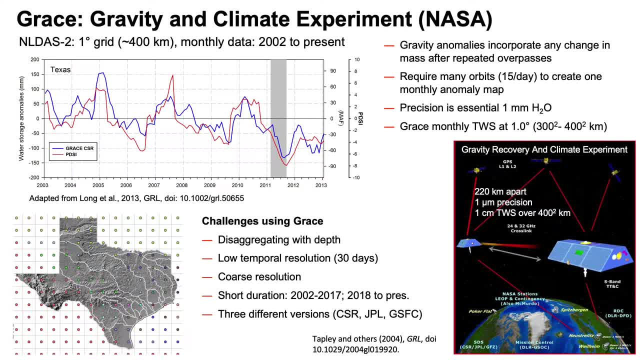 which is too coarse for local or even regional applications. At larger scales, GRACE provides a direct measure of storage anomaly and precipitation needed for recovery. For example, the GRACE data measured a departure of nearly 90 million acre feet during the 2011 drought. 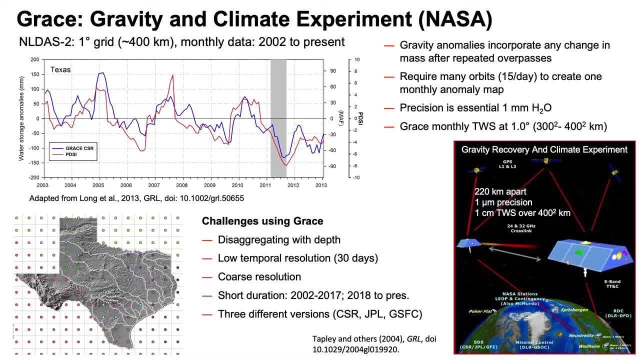 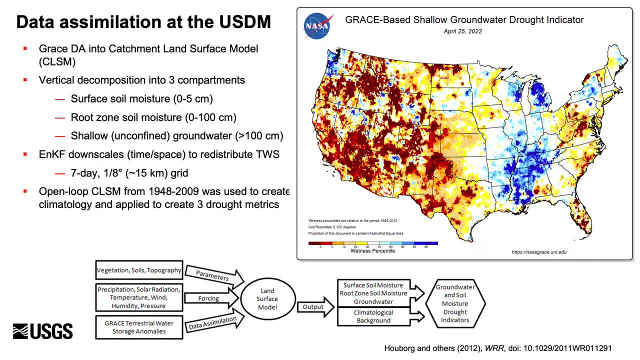 of record in Texas, Nearly 150 millimeters of precipitation would be needed to recover from the drought, which didn't occur until 2015.. In order to increase the temporal and spatial resolution of GRACE data and to isolate groundwater from total terrestrial water storage, 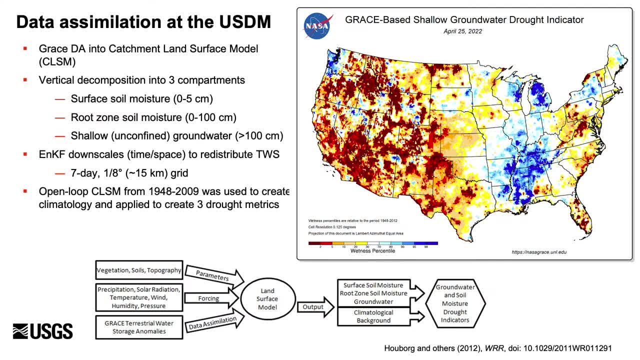 scientists at NASA Goddard Space Flight Center integrated GRACE data with other on-ground and space-based meteorological observations within the catchment land surface model using ensemble common filter or type of data assimilation to increase record length and develop more robust percentiles from relatively short GRACE mission.